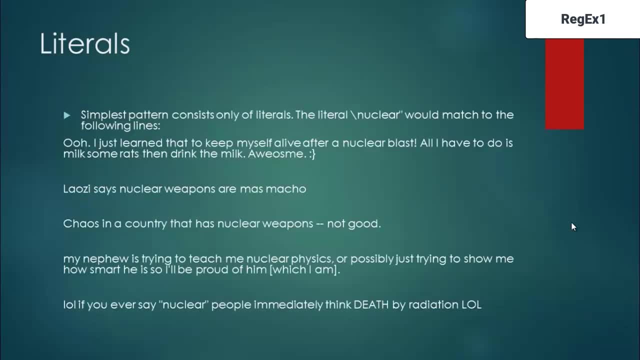 So, moving on, what are literals? So I'm showing the simplest pattern: only literals. Literals are nothing, but you know, you know just a word, a word or characters that matter directly. I have a set of examples here. So, as you can see, there are like multiple texts which have the word nuclear in it, but 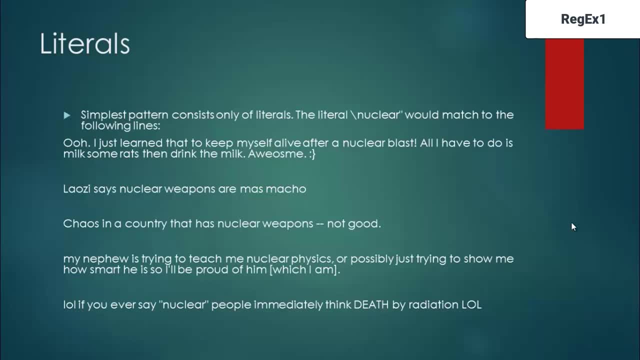 the usage of nuclear is different and the sentiment behind every usage is different. For example, the first line: I just learned that to keep myself alive after a nuclear blast, all I have to do is milk some rats and drink the milk. awesome, So this is think. 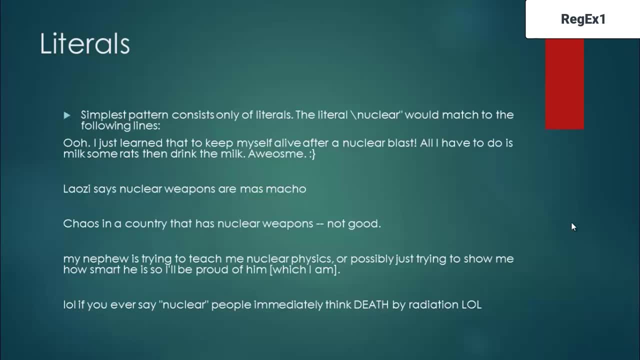 of it as like some kind of a Facebook or a Twitter feed that's coming out. So like the first sentence, you saw someone like making fun of the nuclear blast, So you have the word nuclear. so Lavosy says nuclear weapons are mas macho, So Lavosy some kind of Mexican. 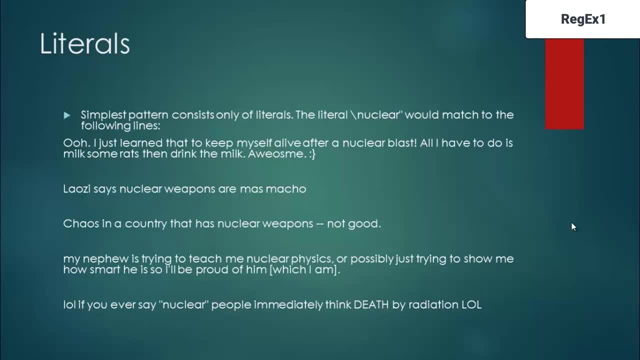 statement where you have the nuclear weapons are. you know it defines the characteristics of a male. So chaos in a country that has nuclear weapons- not good. So this is one more sentence. My nephew is trying to teach me nuclear physics, or possibly just trying. 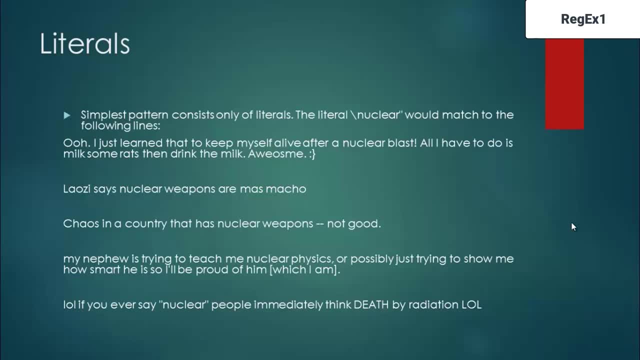 to show me how smart he is, So I'll be proud of him. So, Lord Lull, if you ever say nuclear, people immediately think death by radiation. so you see multiple usages of the word nuclear here. so let's say there is a text, analytics you have to run and 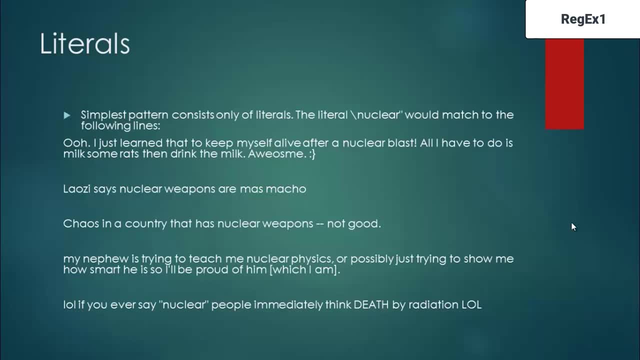 you want to see how many people people are talking about. you know, a nuclear test or a nuclear blast that happened? there cannot be a nuclear blast, but if there is any kind of nuclear test run by any countries and is there someone who is talking on Twitter or Facebook, so as you can see, the word nuclear is spoken. 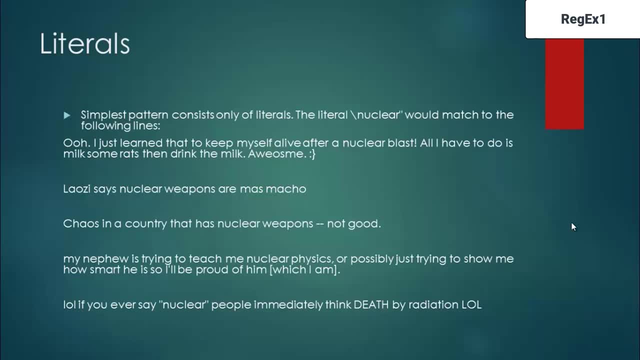 by a lot of people and, as you can see from the text there are, the sentiments are much, much different. so in these your task will be to identify those which talk relatively to do the nuclear test or something like that. so if the problem definition may vary, but here if I use slash nuclear, it will given using our 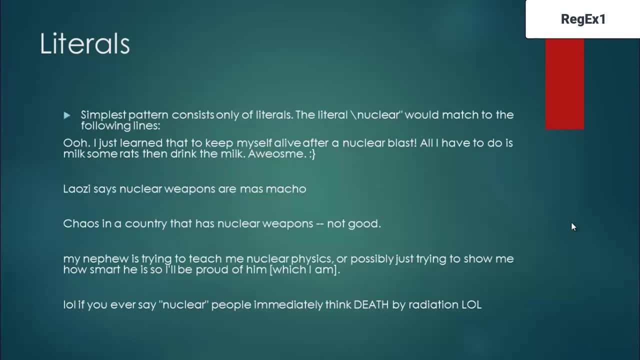 programming, the slash nuclear will match to all these statements and from these statements you can extract the statements that you require from the for your analysis purpose. so it is a simple literal which means nothing, but you are searching for the text nuclear, that's all. you're just searching for nuclear, and if it is found in that, it will. 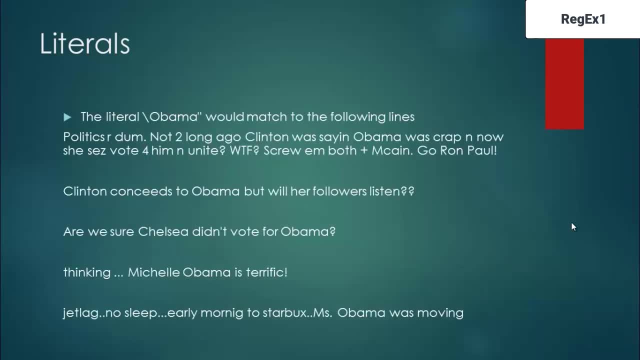 return a positive match. so, again, I extracted these examples from online. so, as you can see the next literal Obama, so would match you can see the next literal Obama, so would match to the following lines. so, for example, there is a. you can see, as these will be. 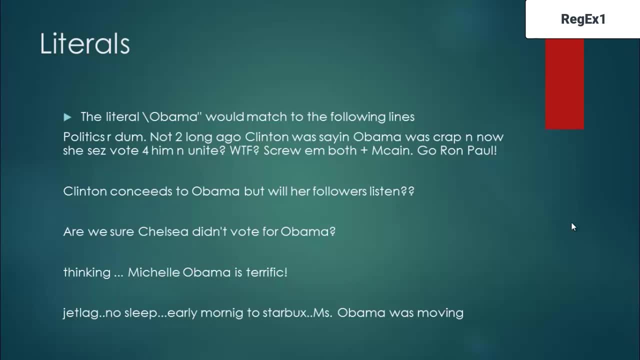 like Facebook or Twitter feeds. politics are dumb. not too long ago, Clinton was saying Obama was crying, now she's vote for him and unite WTF. screw them both, plus McCain. go Ron Paul. so this is some kind of a Facebook or Twitter feed. the baron user is showing his anger towards Obama, so now Clinton concedes to Obama. 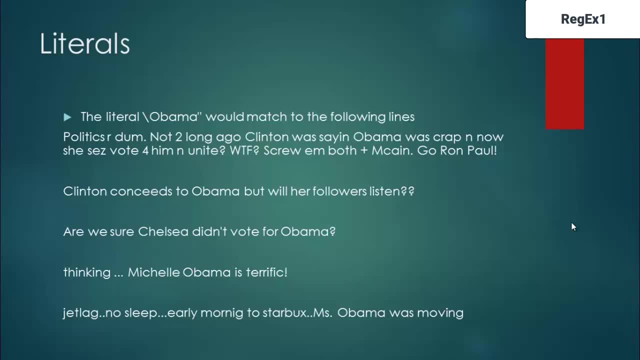 but will follows listen. so, Clinton, as they talking about Hillary Clinton. so that's the reason we are talking about Hillary Clinton, so that's the reason we are getting. will her followers listen? are they sure? tells he didn't vote for Obama, thinking Michelle Obama is terrific jet lag. no sleep early morning. 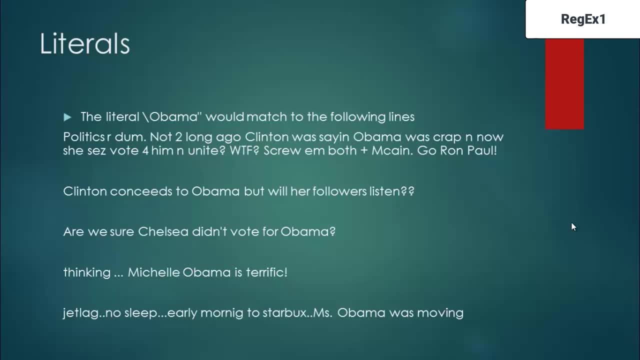 to Starbucks. mr Obama was moving. so again here also you found a lot of statements reading room Obama. so if there is an analysis where you want to find how the people who are talking about Obama and their sentiments, you need to perform a sentimental analysis so you can move on to. 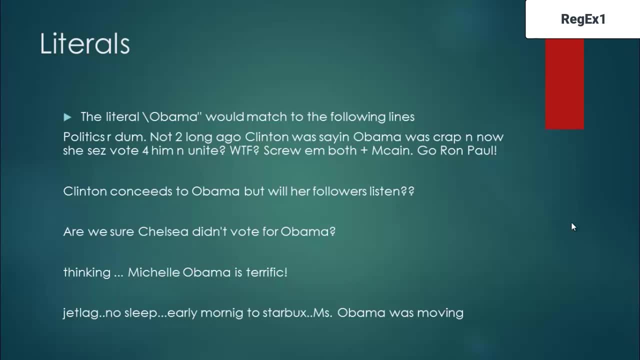 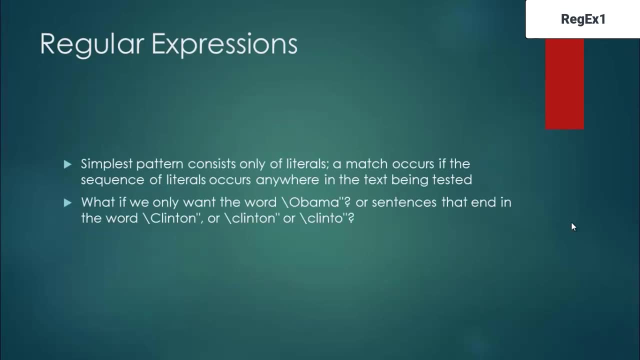 use the simple little Obama will being give you all these sentences where the word Obama was used now. so the simplest pattern that I showed you- for nuclear and Obama are best examples- which contains only of literals. a match occurs if the sequence of literals occurs anyways in the text being tested. 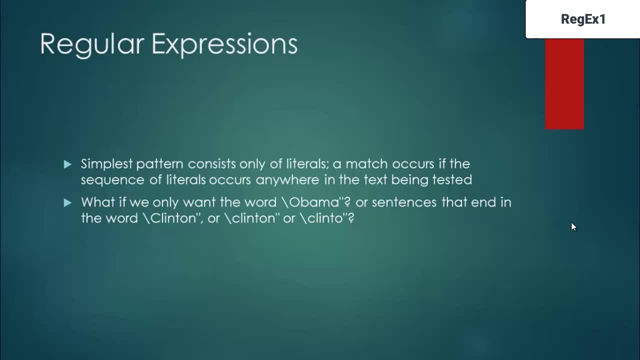 what if we only want the word Obama or sentences that in the word Clinton, sentences that end in the word Clinton? so I'm being specific here. where I want the sentence that ends with Clinton, the last word is Clinton or Clinton or Lento, with a capital C, with a small C and n being removed in the end. so if I